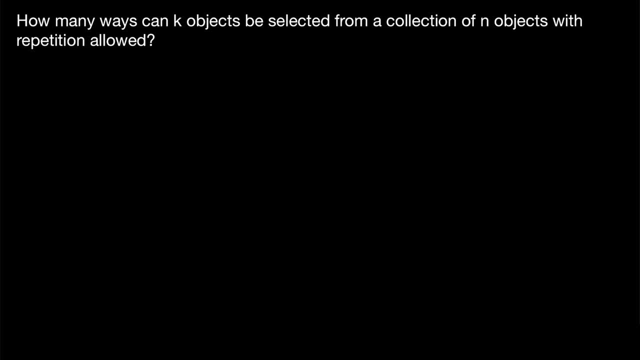 monthly donation. there will be a link down in the description And be sure to leave your video requests down in the comments. Usually when we begin to count combinations, we do not allow repetition. You may recall that the number of ways k objects can be selected from a collection. 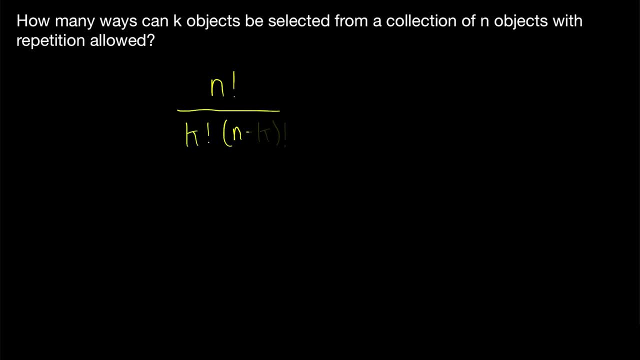 of n objects is equal to this n factorial divided by k factorial times n minus k factorial. Again, that's the number of combinations of k objects that can be selected from a collection of n objects. It's denoted like this: This is read: n choose k and it's called a binomial. 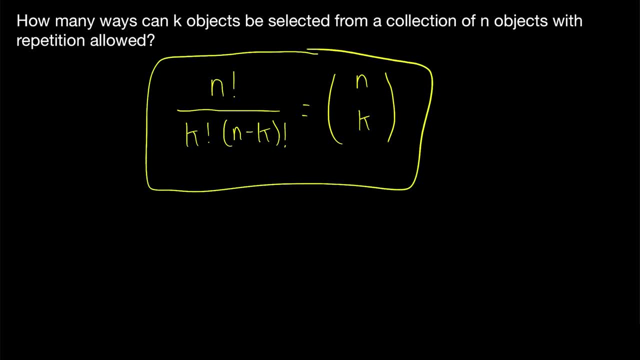 coefficient. You should already be familiar with this sort of thing. before tackling today's problem, I'll leave links in the description to lessons all about this. combinations without repetition- Also the problem of counting combinations without repetition and the problem of counting combinations with repetition. both of those can be phrased in terms of counting subsets. 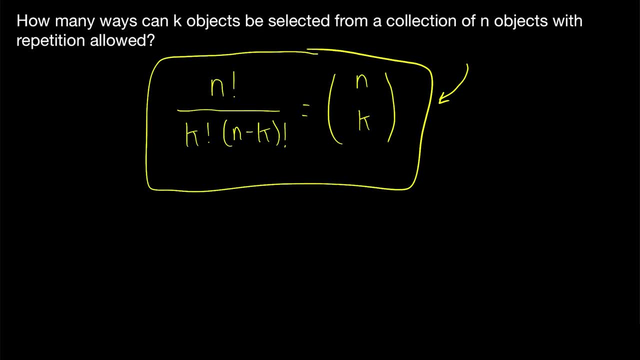 of sets and multisets. But in the interest of time today, we're pretty much going to not touch on the set formulations of these problems. Just remember: when we're counting combinations, we're not worried about the order of the objects we're selecting, which is why sets and subsets. 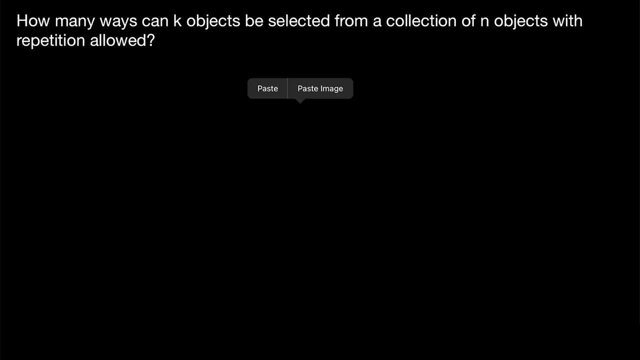 work well to represent these problems. All right, no more dilly-dallying. Let's go over a very cool solution to this problem. Let's say we've got this collection of n objects- a1,, a2, all the way. 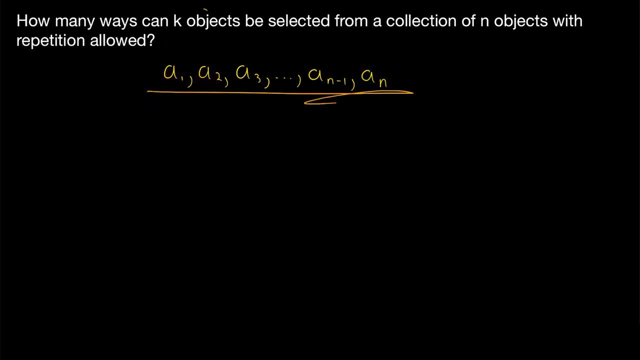 through an Suppose that I've selected k of these objects And repetition is allowed, so I've probably selected some of the objects multiple times. How could I communicate the combination of objects that I selected to you? One way is like this: I 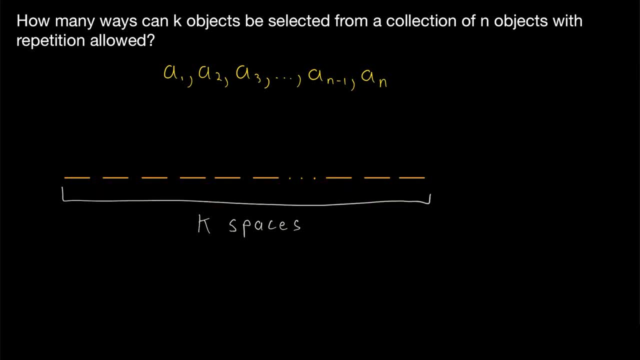 could say: here are k spaces and I'll fill them in with the objects I selected. And since order doesn't matter, maybe I'll be nice and list the objects in the most convenient order. So if I selected any a1s, I'll put the a1s first, Then I'll put the a2s and then I'll put the a1s And. 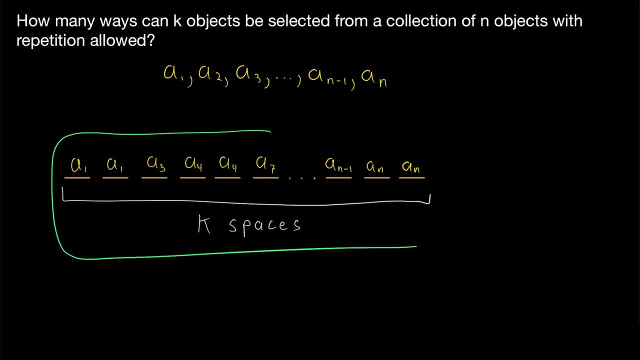 then here you go. I've written out all the k objects I selected. You see, I selected two a1s, one a3,, two a4s and so on, And this just describes one of the many ways that I could select k objects from our collection of n objects, with repetition allowed, And perhaps this seems a. 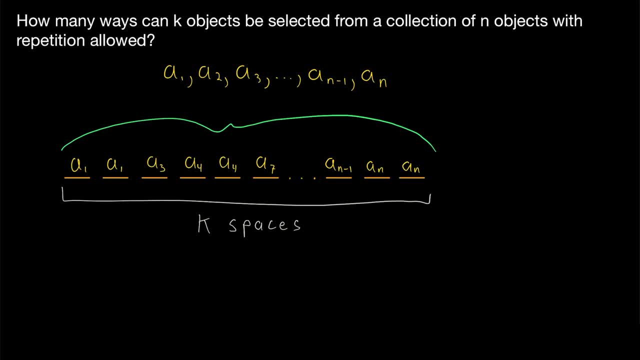 bit daunting how we could possibly count the number of ways to fill in these k spaces with selection of n objects, with repetition allowed. And so I've written out all the k objects I selected. And then here you go: I've written out all the k objects I selected. You see, I selected. 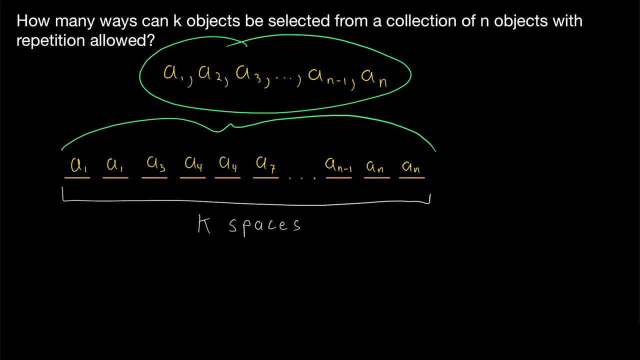 n objects with repetition allowed, And so I've written out all the k objects I selected, And so I've written out all the k objects I selected, And so I've written out all the k objects I selected of these n objects. especially because repetition is allowed, We might wonder: is there another way? 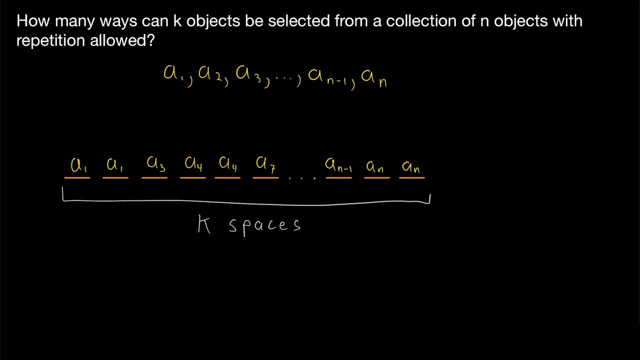 I could completely communicate the combination of objects that I selected without literally writing out every single one. Here's an idea. Maybe I give you these k spaces, but I draw bars separating the different sections that I want to be filled with different types of objects. 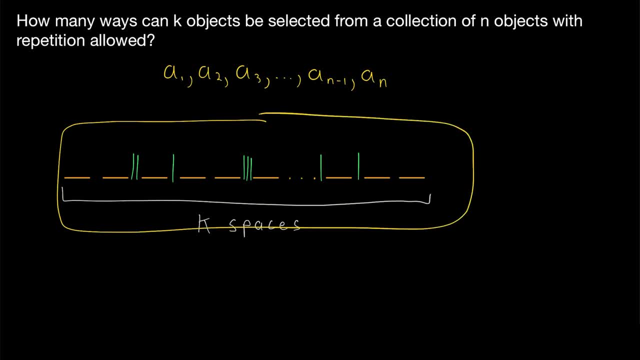 And so I give you this. I've placed a bar everywhere. I want you to stop placing one object and move on to the next. Let's try filling this in to make it more clear what I mean. We begin with the a1s and we see there are two empty spaces where we can place. 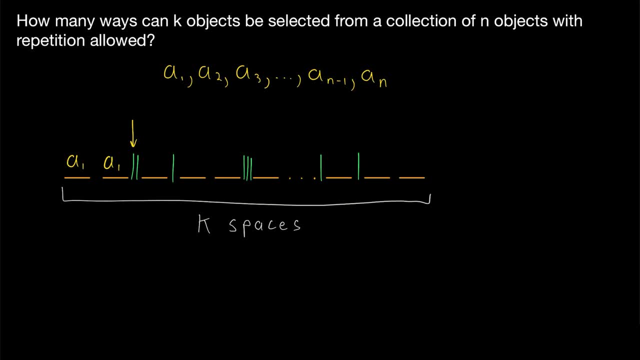 the a1s. But then we encounter a bar, which means I want you to stop placing the a1s and move on to the a2s. But then we have another bar, which means I want you to stop placing the a2s and move on to. 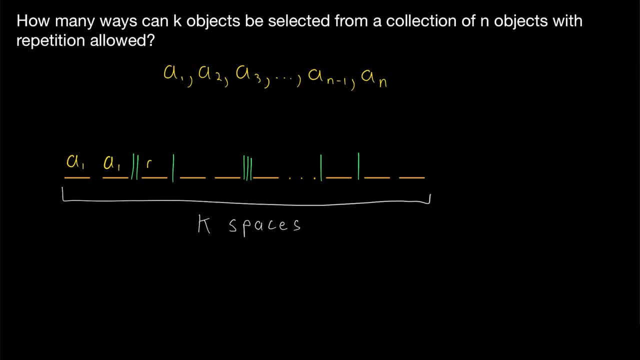 the a3s, So I don't want any a2s. Then we have another bar, which means I want you to stop placing the a3s, And then we have a space for an a3, and another bar to say stop placing the a3s and 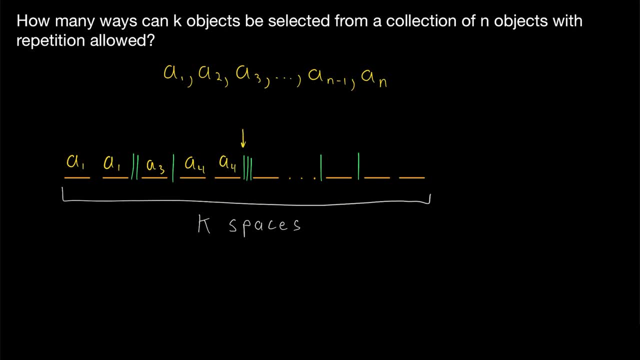 move on to the a4s. Then we have a bar to indicate we should stop placing the a4s, then another bar to indicate we should stop placing the a5s, and then another bar to indicate we should stop placing the a6s. So then we're on to a7. And we'd continue in the same way. The bars have completely described. 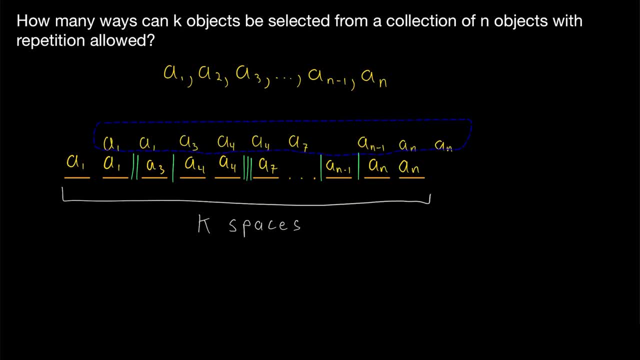 the collection of objects that I listed out earlier. I'm pasting it, We can see. it's the same thing. Then. my point to you is that to count the number of ways we can select k objects from a collection of n objects, with repetition allowed, to count. 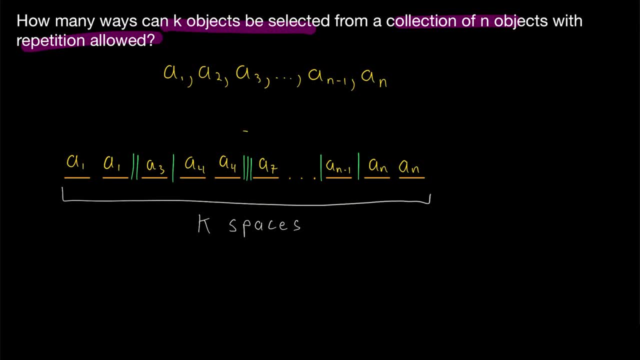 that we can just count the number of ways that we can place bars in spaces. to put it simply, Because each combination of k objects corresponds to exactly one arrangement of these bars and each arrangement of these bars describes exactly one combination of k objects. So, between the k objects that we're placing and all of these, 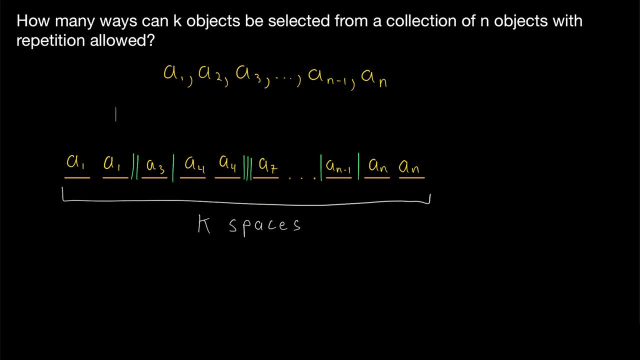 bars. how many things do we have total? Well, we've got the k spaces and then we have n-1 bars. We have n-1 bars because we have n objects total and we place a bar to indicate where we should. 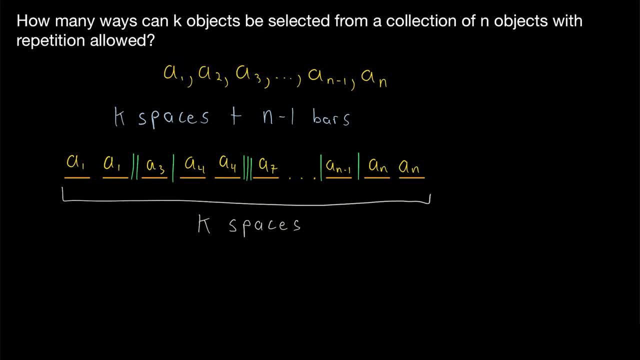 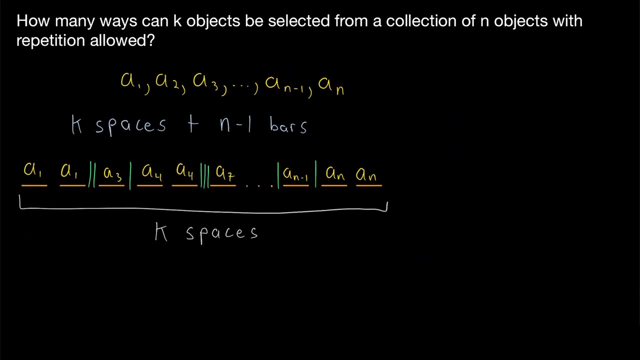 stop placing each object, Except for a n. We don't need a bar to indicate where we should stop placing the last object, because we can just stop when we run out of spaces, since it's the final object. And so we can answer the question by imagining we have a total of k plus n-1 spots. to put things, 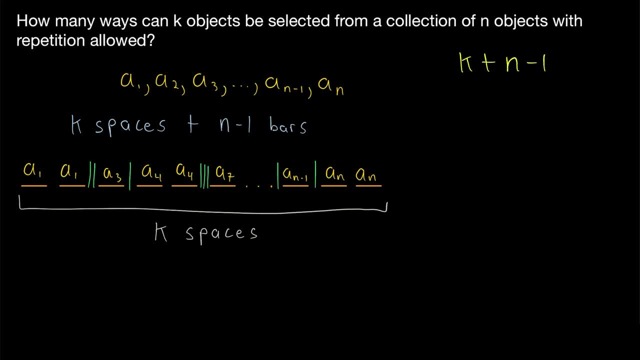 Again, that's k plus n-1 spots. to put things, We're going to have k objects and we're going to have n-1 bars. So to count the number of combinations of k objects from a collection of n objects, with repetition, 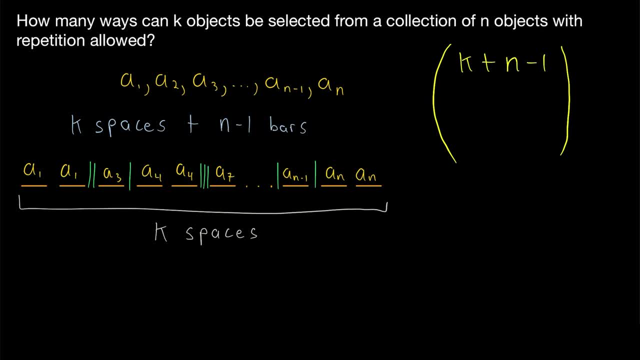 allowed. we just need to count the number of ways that we can place n-1 bars in a total of k plus n-1 spots And that, my friends, is just k plus n-1. choose n-1.. And that is the answer. So once, 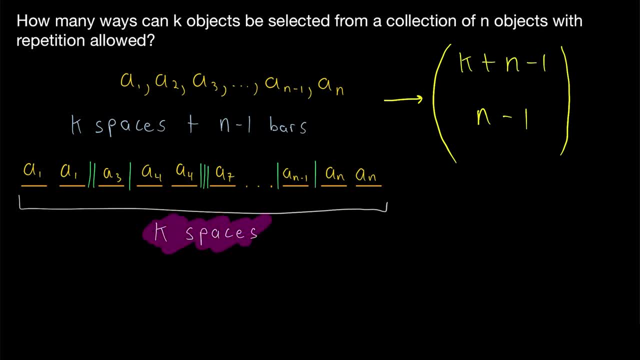 more. instead of just having k spaces, we can just place n-1 bars in a total of k plus n-1 spots. We can think of it as having a total of k plus n-1 spaces, so that we have a space for the bars as. 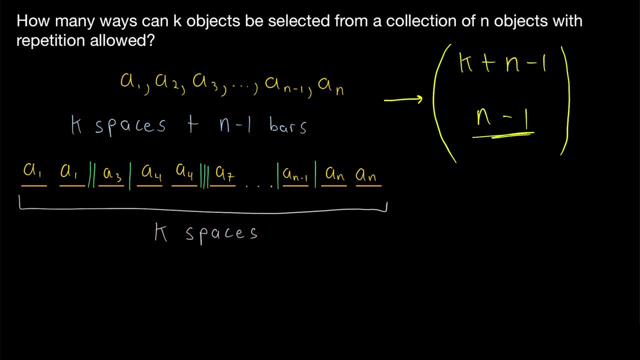 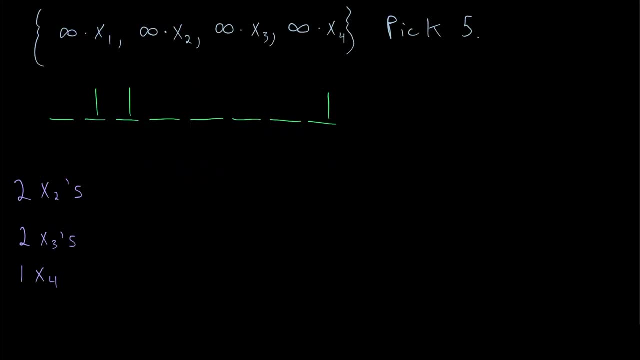 well, And then the number of ways that we can pick n-1 spaces for our bars from those k plus n-1 spaces is the number of combinations of k objects from a collection of n with repetition allowed. Now let's just see quick two examples to further convince you of this correspondence between a. 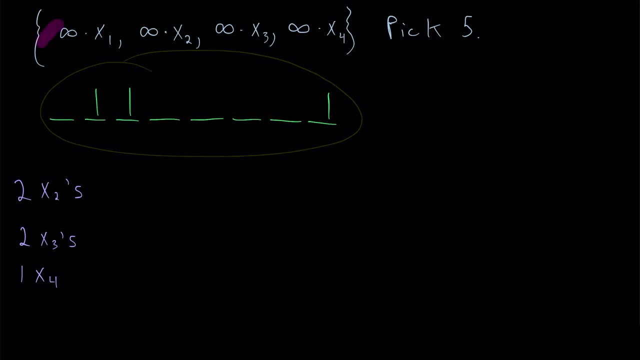 combination of objects and spaces. Here we've just got one way of representing a multi-set. This set has objects x1,, x2,, x3, and x4, and it has infinitely many of all of them. So we want to pick 5, and of course we're allowed. 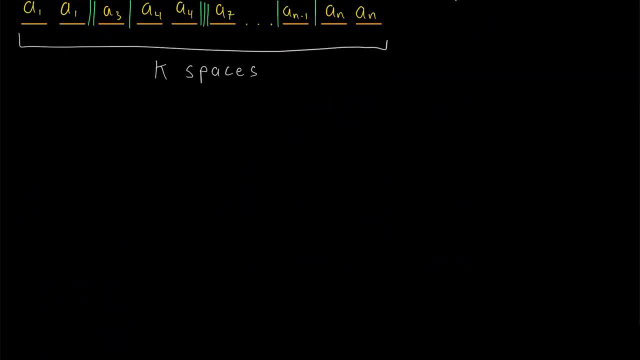 to pick the same one multiple times. Remember we should have a total of k plus n-1 spots or spaces. k is the number of objects we're picking- in this case 5, and n is the number of different objects we have to choose from. We have 4 different objects to. 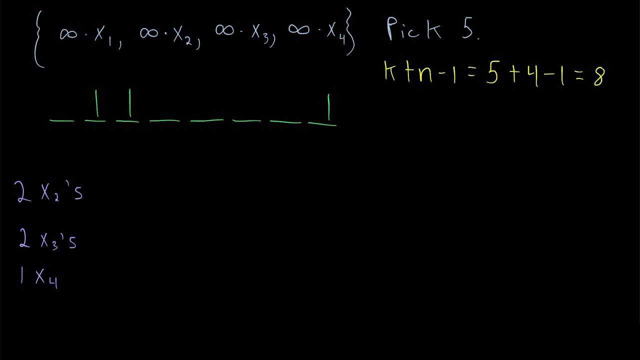 choose from. So 5 plus 4 minus 1, that gives us 8.. Here we have 8 spaces that have n-1, or 3, bars placed in them Because, remember, we are picking n-1 spaces for the bars. So in this case, 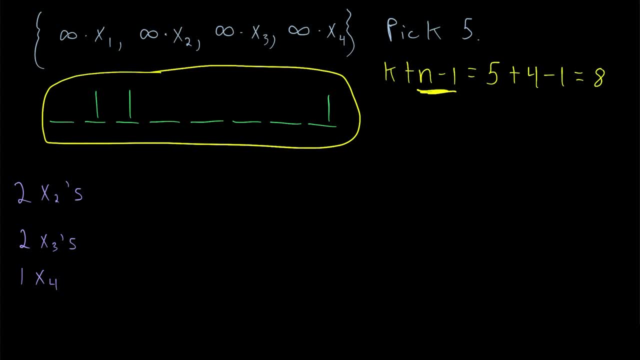 n-1 is 3,. we've got 3 bars in the 8 spaces. How does this describe a combination of 5 of these objects? Well, we begin with the x1s. There's one space for an x1,. 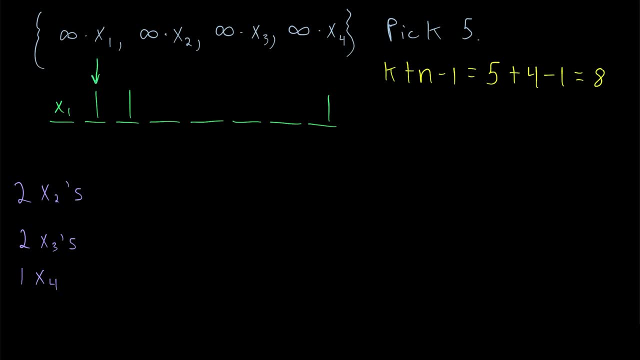 then we encounter a bar, So we stop with the x1s and move on to the x2s. Then we encounter another bar, so there won't be any x2s and we move on to the x3s. We've got a lot of spaces for these x3s. 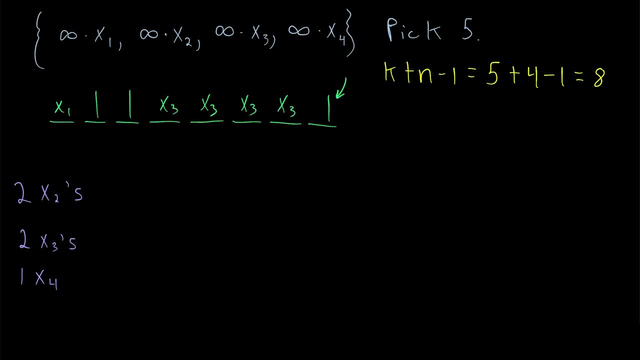 and then we encounter a bar that says: stop with the x3s, move on to the x4s. but there are no more spaces. so we're done, So we've got a lot of spaces for these x3s. and then we encounter a bar. 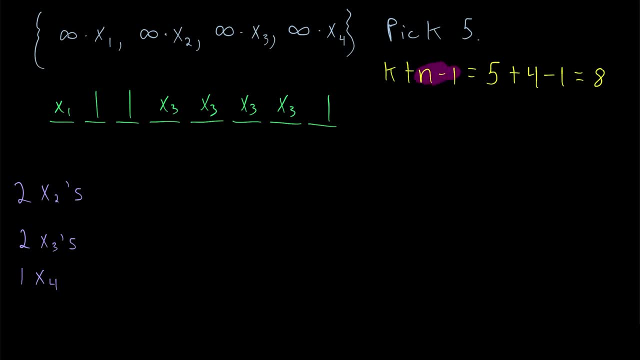 So again, the point is to just make clear how placing n-1 bars in k plus n-1 spaces describes a combination of our objects with repetition. Quickly, let's just go in the other direction. for this example, We're told that our collection has 2x2s, 2x3s and 1x4.. How can we? 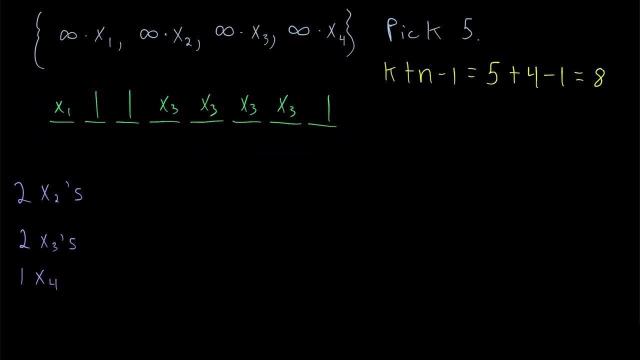 use the spaces and the bars to represent this combination of objects. Well, again, we should have k plus n-1s. and then we encounter a bar that says: stop with the x2s, move on to the x3s. and then we encounter a bar that says: stop with the x3s, 2x3s. and then we encounter a bar that says: 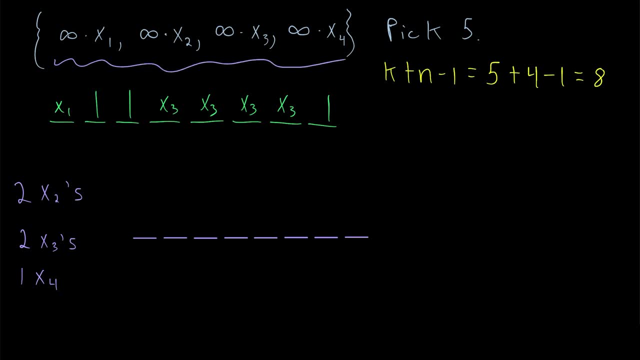 k plus n-1 spaces and we're picking from the same collection of objects. so this is still equal to 8, and we have 8 spaces. Then we just need to place n-1, or 3 bars within the spaces. 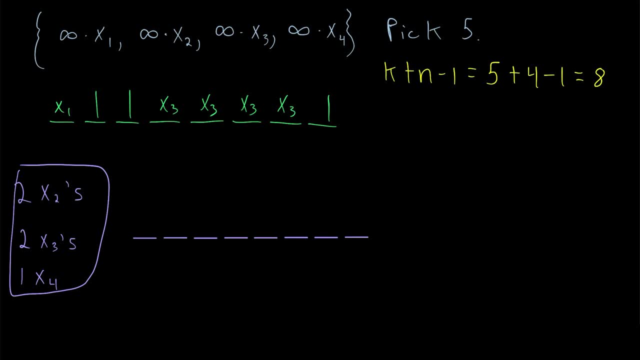 We see that we haven't selected any x1s, so we need the first space to have a bar That says immediately stop with the x1s and move on to the x2s. Then we have 2x2s, so those would take up. the next 2 spaces, and then we would have a bar that says stop with the x1s and move on to the x2s. Then we have 2x2s, so those would take up the next 2 spaces, and then we would have a bar. 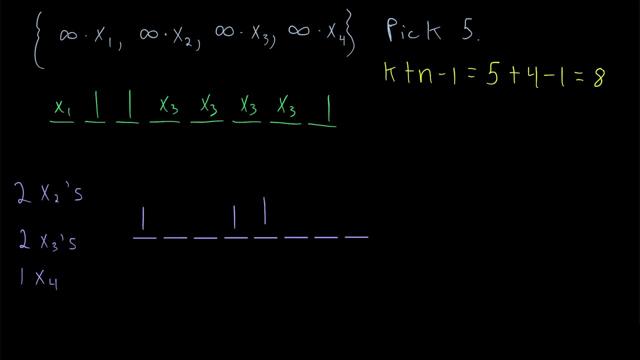 to indicate that we should move on to the x3s. x3s would take up the next 2 spaces again, and then we would place a bar to indicate that you should move on to the x4s, And then there's one space left for the 1x4.. Again, we don't need a final bar, because that's the last space. 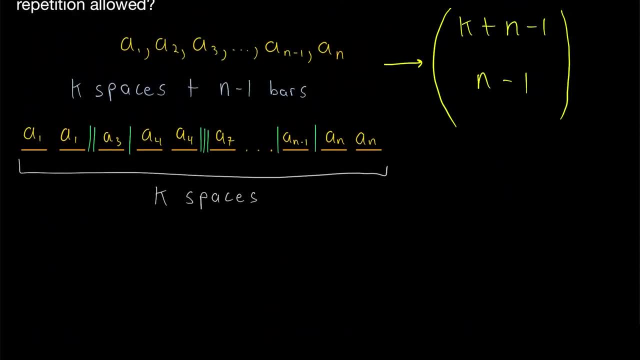 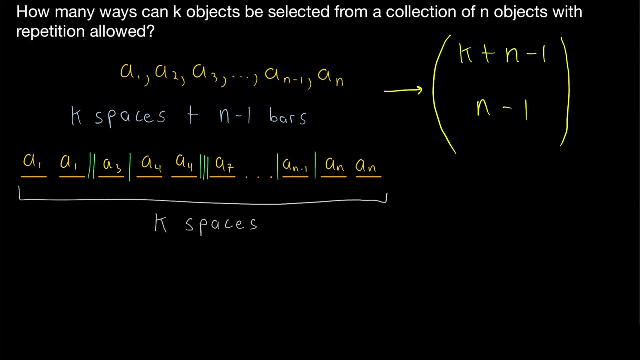 so we know that's the end. So hopefully that helps to convince you that the number of ways we can place n-1 bars in k plus n-1 spaces is indeed the number of ways that k objects can be selected from a collection of n objects with repetition allowed. and that's pretty sweet. But 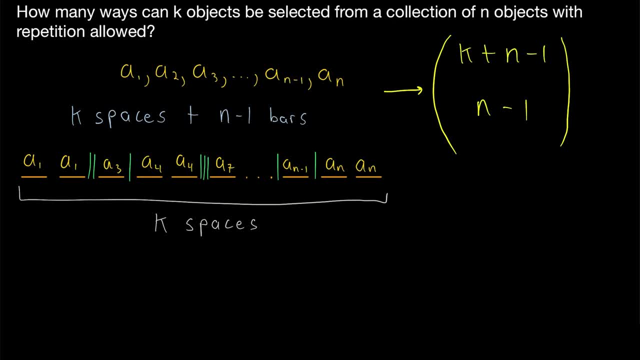 it gets even better By the symmetric property of binomial coefficients and I'll leave a link in the description to a proof of that property. k plus n-1- choose n-1 is equal to k plus n-1- choose k, which I think you'll agree is a bit nicer. So the number of ways that k objects can. 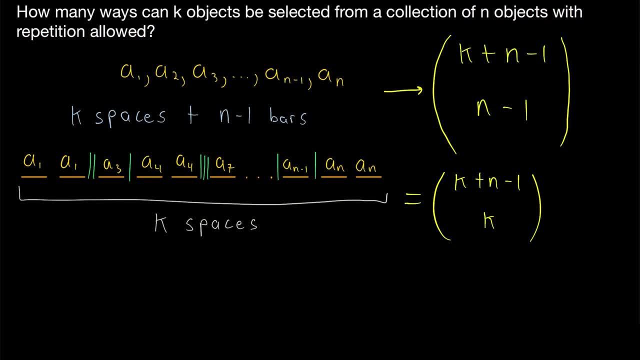 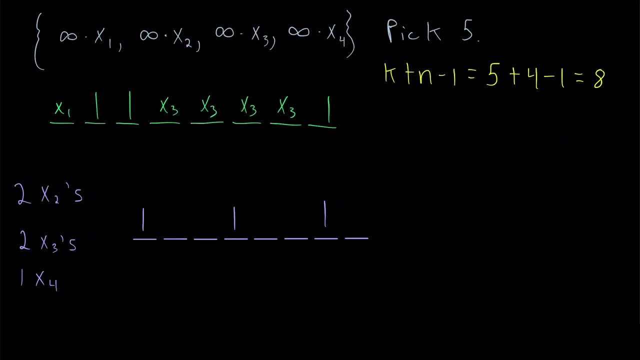 be selected from a collection of n objects with repetition allowed. is k plus n-1. choose k. Who'd have thought? Finally, let's go back to these examples to actually do the calculation. How many ways can we pick 5 objects from these 4 distinct objects, If repetition 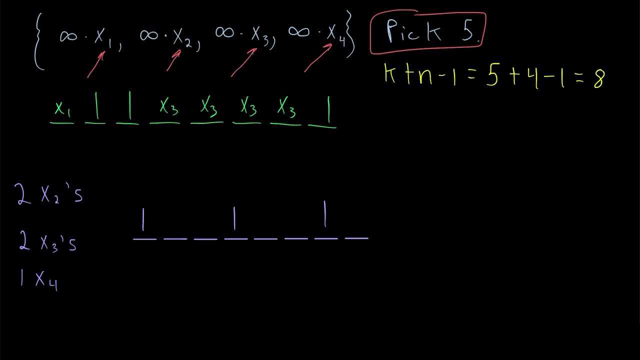 wasn't allowed, of course, there would be no ways to do it. You can't pick 5 objects from a collection of 4.. But since we're allowed repetition, we can use the beautiful expression that we just explained. The answer is this: We have a binomial coefficient: the number of objects. 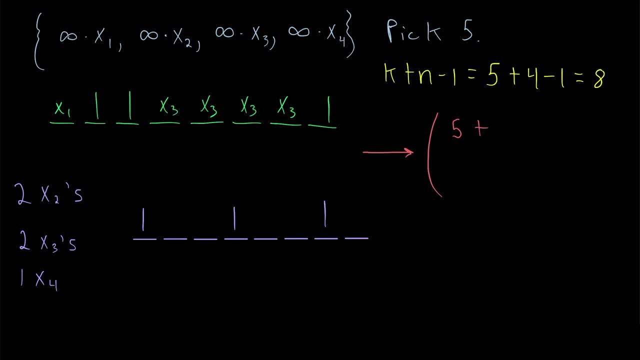 we're selecting, which is 5,, plus the number of distinct objects we have to choose from, which is 4 minus 1, and then choose 5, the number of objects we're selecting. That, of course, is equal to 8.